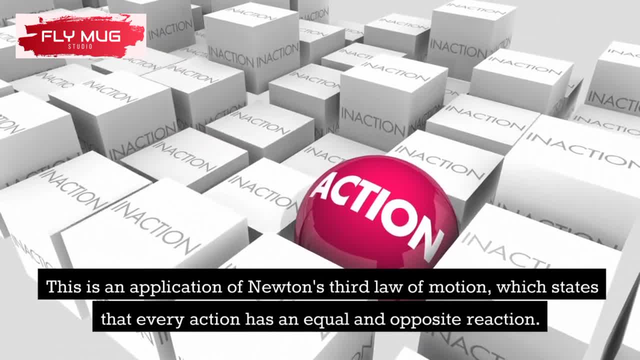 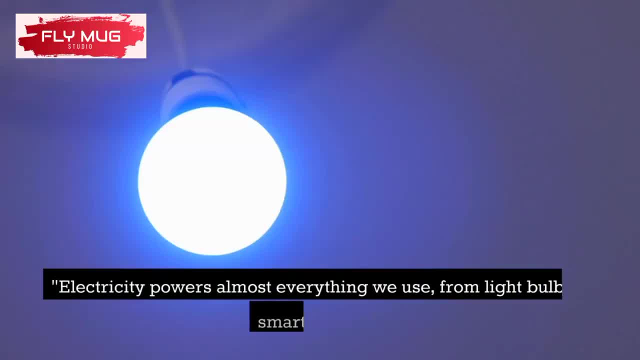 which is the law of motion. The law of motion states that every action has an equal and opposite reaction. As you push the pedals, the bike exerts an equal and opposite force on you, allowing you to move forward. Electricity powers almost everything we use, from light bulbs to 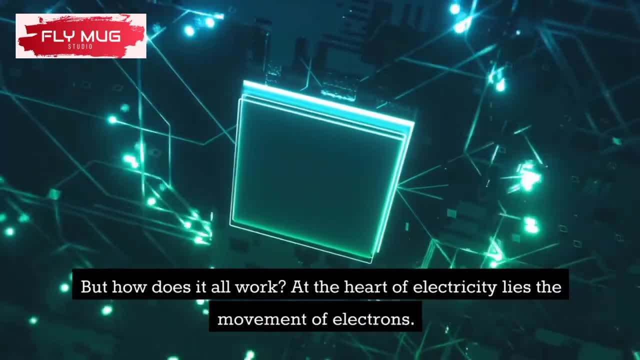 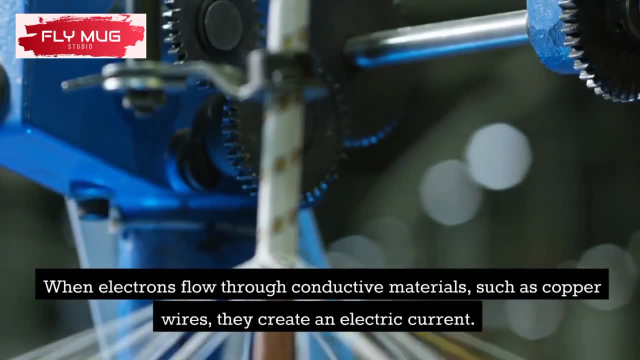 smartphones. But how does it all work? At the heart of electricity lies the movement of electrons. When electrons flow through conductive materials such as copper wires, they create an electric current. This flow of electrons enables the functioning of electrical devices. When electrons flow through conductive materials such as copper wires, they create an. 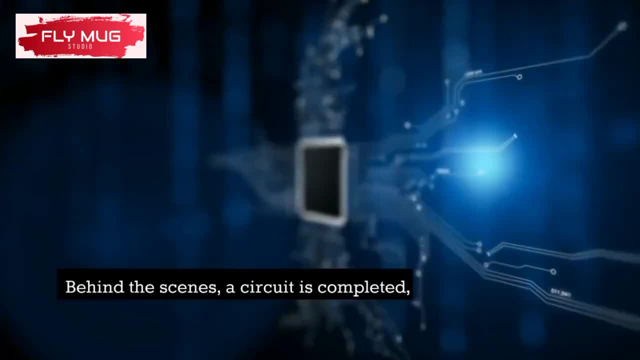 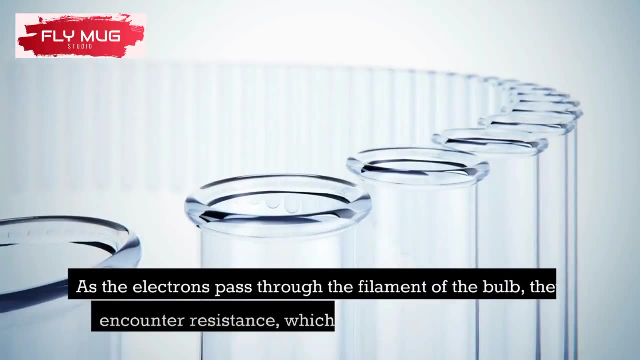 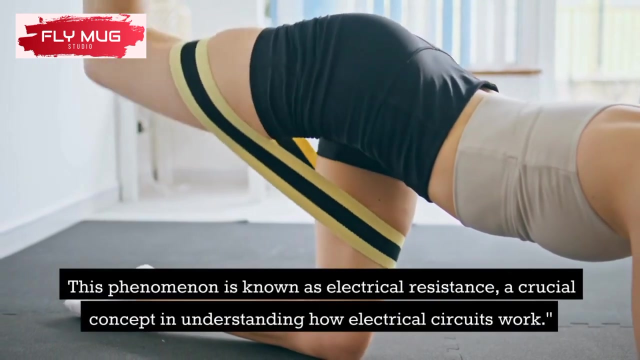 electric current. Imagine you turn on a light switch. Behind the scenes, a circuit is completed allowing the flow of electrons from the power source to the light bulb. As the electrons pass through the filament of the bulb, they encounter resistance which produces heat and light. This phenomenon is known as electrical resistance. 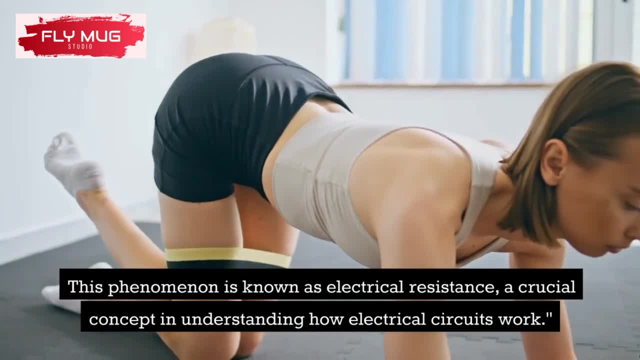 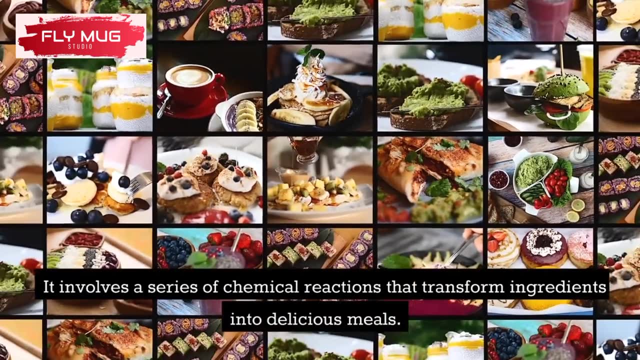 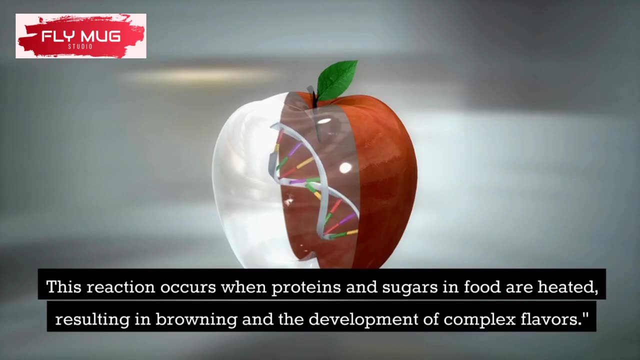 a crucial concept in understanding how electrical circuits work. Cooking is both an art and a science. It involves a series of chemical reactions that transform ingredients into delicious meals. One such reaction is the Maillard reaction. This reaction occurs when proteins and sugars in food are heated, resulting in browning and the development of complex flavors. 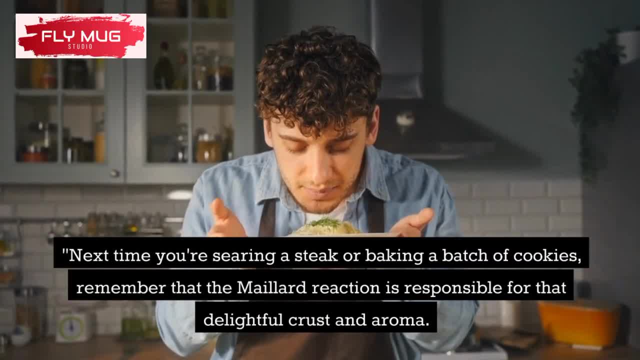 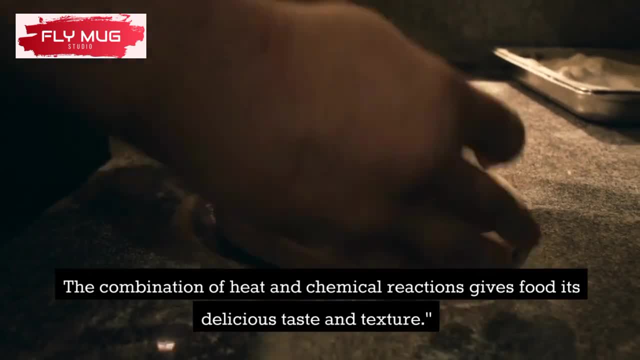 Next time you're searing a steak or baking a batch of cookies, remember that the Maillard reaction is responsible for that delightful crust and aroma. The combination of heat and chemical reactions gives food its delicious taste and texture. Breathing is essential for our survival. 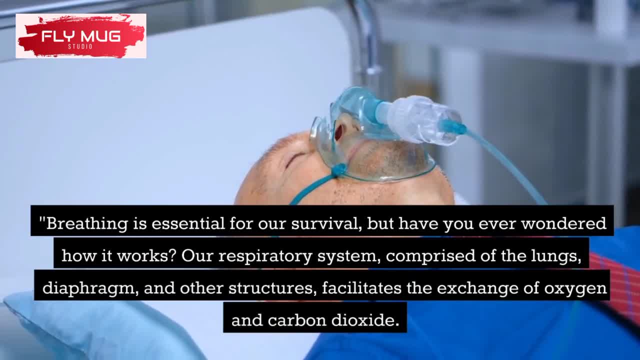 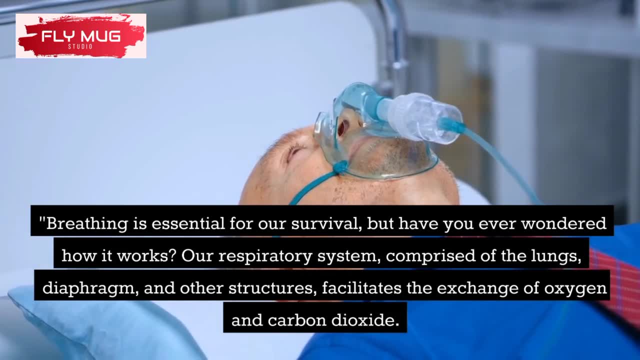 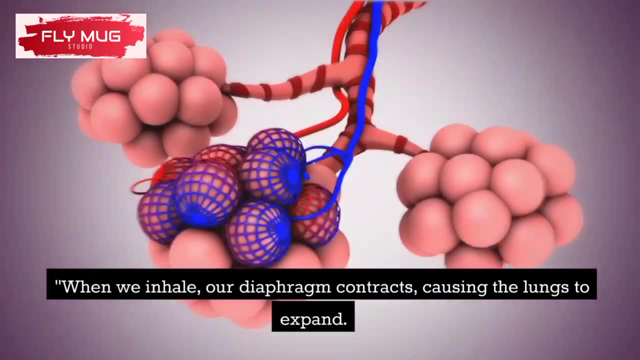 but have you ever wondered how it works? Our respiratory system, comprised of the lungs, diaphragm and other structures, facilitates the exchange of oxygen and carbon dioxide. This process is known as respiration. When we inhale, our diaphragm contracts, causing the lungs to expand. This expansion creates a 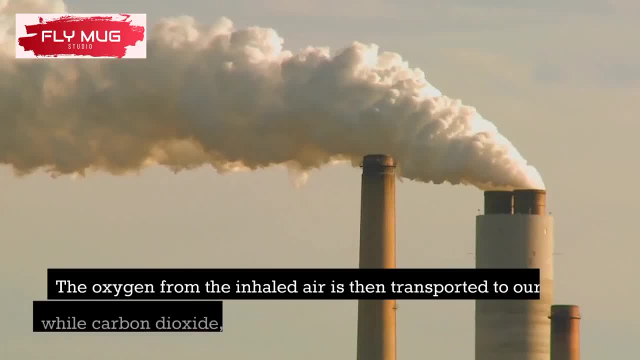 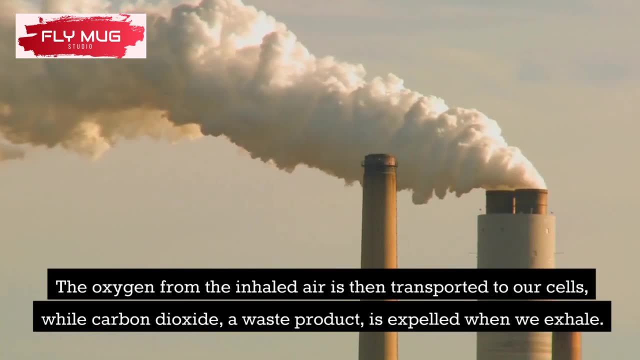 pressure difference that draws air into our lungs. The oxygen from the inhaled air is then transported to our cells, while carbon dioxide, a waste product, is expelled when we exhale. This intricate process ensures our body receives the oxygen it needs for energy production. 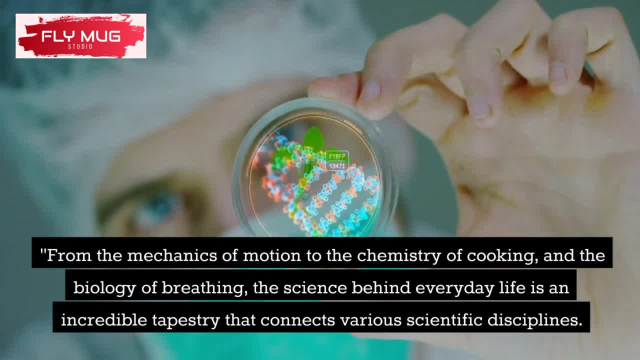 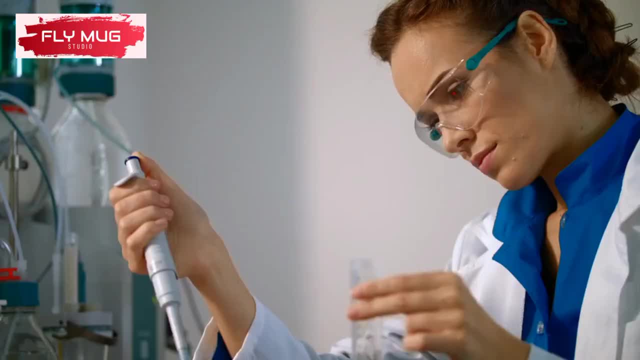 From the mechanics of motion to the chemistry of cooking and the biology of breathing. the science behind everyday life is an incredible tapestry that connects various scientific disciplines By understanding these scientific principles.